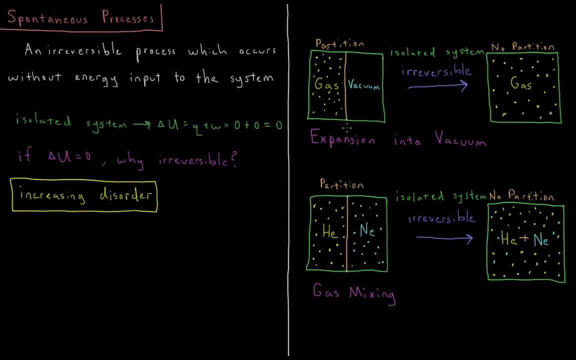 Half of it is vacuum and there's a partition which separates the gas and the vacuum. So this is an isolated system, so there's no change in energy from the outside of this system. Now let's say what happens when we remove this partition. Well, we instinctively know that this gas is going to expand to fill up the entire container, So this gas is going to expand into the vacuum. Now the vacuum is defined as the absence of gas. 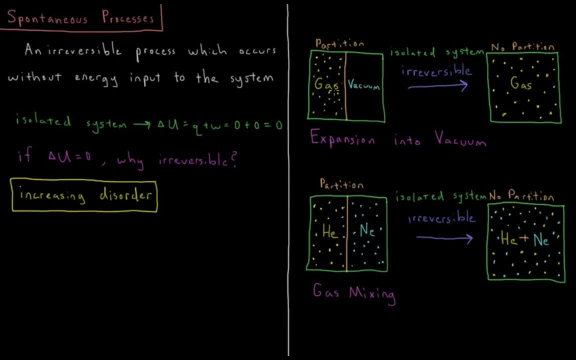 So there's no pressure here. So the external pressure that our gas is expanding against is zero. So there's not any work that's being done during this expansion event. So there's no work And the vacuum doesn't have any energy. It's the absence of particles, So there's no heat to transfer to or take away from the vacuum. So no heat transfer occurs in this process. So the total energy change that occurs during this process of the gas expanding into a vacuum is zero. 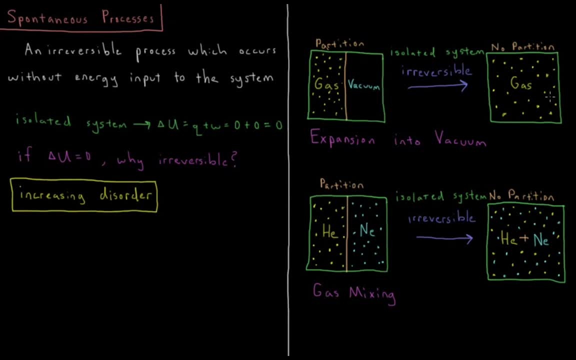 So we know that the gas spontaneously expands into the vacuum, but it will not spontaneously create a vacuum out of itself again. So we know that this process is irreversible. but since the change in energy is zero, why is it irreversible? What is it that's the defining characteristic of this system that causes this process to occur in this direction, but not in the reverse? 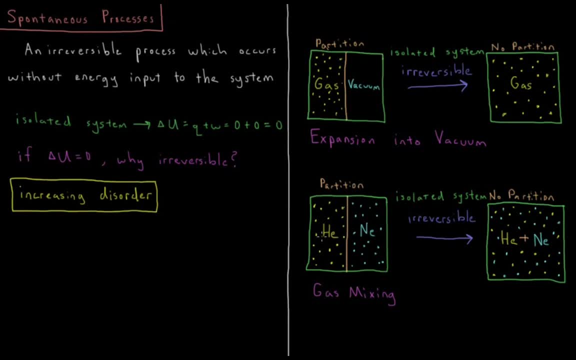 So similarly, we can look at the bottom situation here. We have two gases, so helium and hydrogen. We have helium on the left, neon on the right, both at pressures where they're behaving virtually ideally. So if we have a partition between them and they're perfectly segregated on the left and on the right, then we remove the partition, then the two gases will both expand to fill the entire volume of the system and they'll mix thoroughly. There will be no time at which it returns to being all helium on one side and all neon on the other. It's thoroughly mixed from there on until the end of time. 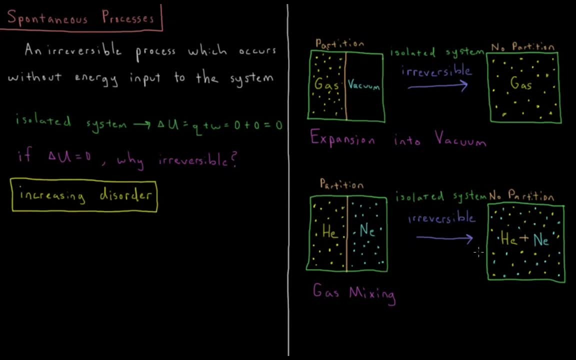 So why is it that this system- again, it's not doing any work to mix together? There's no heat that occurs from mixing. These are ideal gas particles. So what is it that is the defining characteristic that results in both of these being irreversible directional processes in these isolated systems?